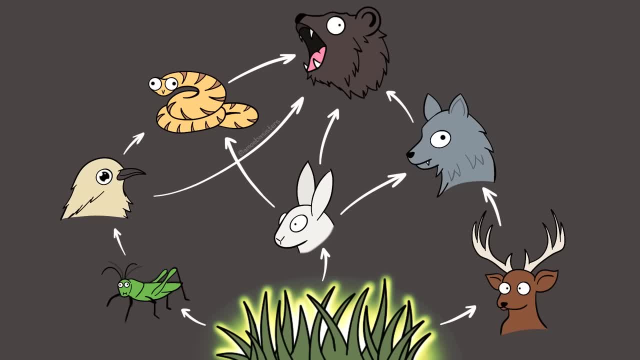 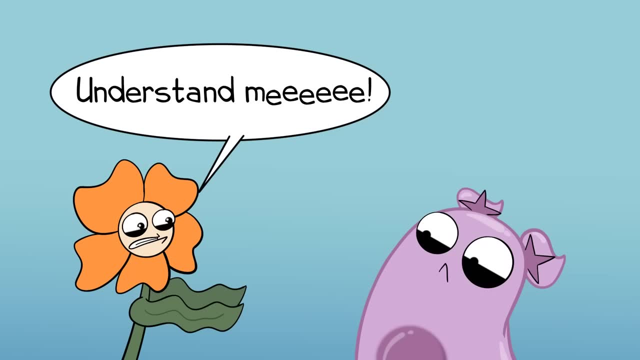 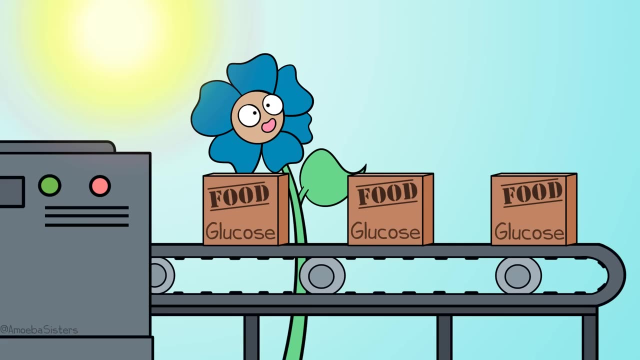 are major producers, Making them indispensable in food webs. Many of our medications and foods come from plants. We need plants, so understanding the nature of the process that plants use to make their own food is paramount. So when I say make their own food, I'm talking about making a sugar that they need specifically. 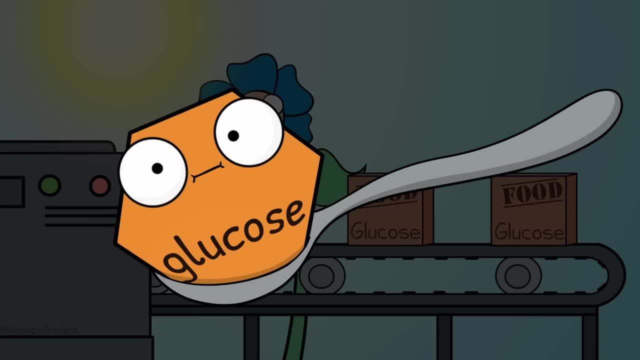 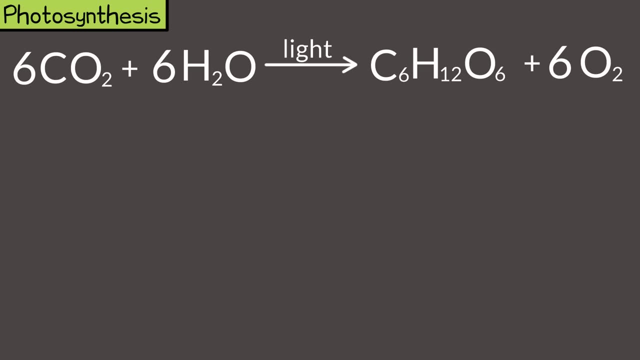 glucose. You need glucose too, but you get it from what you eat. Plants, however, get to make their own glucose in photosynthesis. Here is the balanced overall equation. So photosynthesis has an application similar to what you'll find in many introductory. 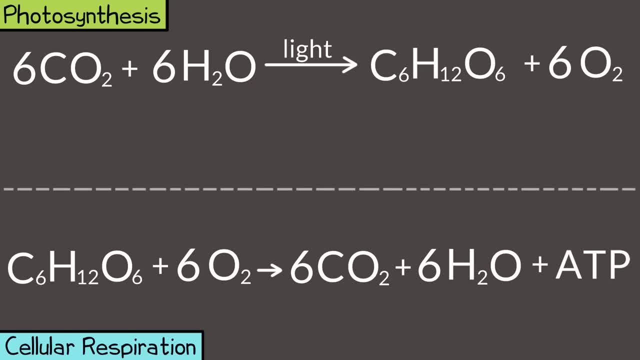 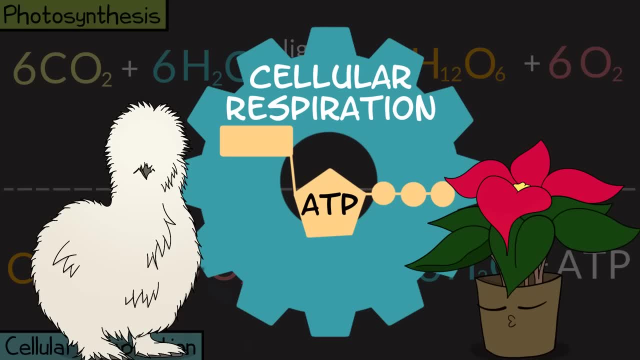 biology textbooks. As you'll notice, it has similarities to aerobic cellular respiration. Recall that cellular respiration is used to make ATP, which is an energy currency, and it's done by plants as well as animals and a lot of other organisms too. 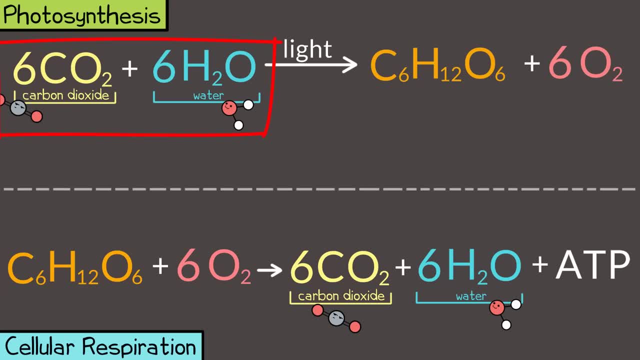 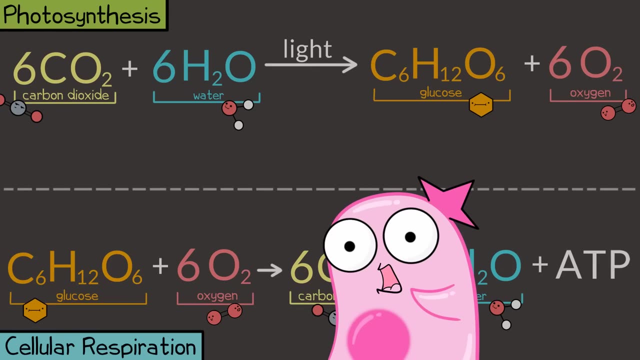 You can see how these reactants inputs of photosynthesis are included in the products outputs in cellular respiration, And the products outputs of photosynthesis are include it in the reactants inputs of cellular respiration. While this doesn't mean that they're simply reversed, it is interesting to see what they have in common. So while both plants and animals need glucose for cellular respiration, plants don't have to be in search of glucose, because they make it. Plants have adaptations to carry out photosynthesis in a variety of environments. One thing plants have to do is capture light. 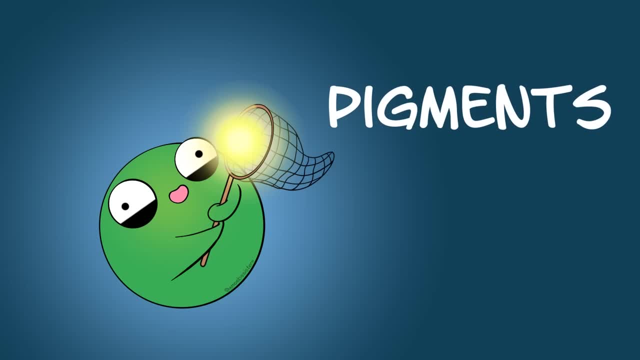 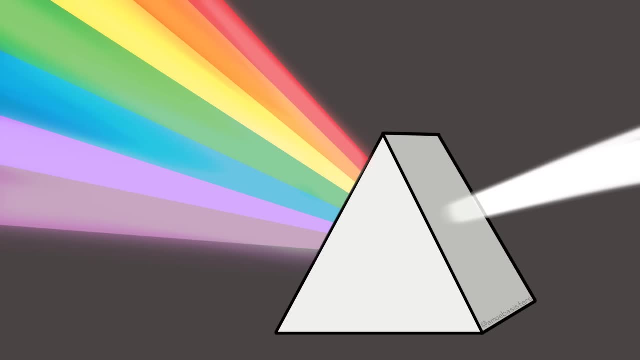 Plants can use light capturing molecules called pigments. Recall that visible light has different wavelengths and those different wavelengths of light have different colors. If you've ever played with a prism before, you can see how light can be separated into a rainbow of colors due to different wavelengths. 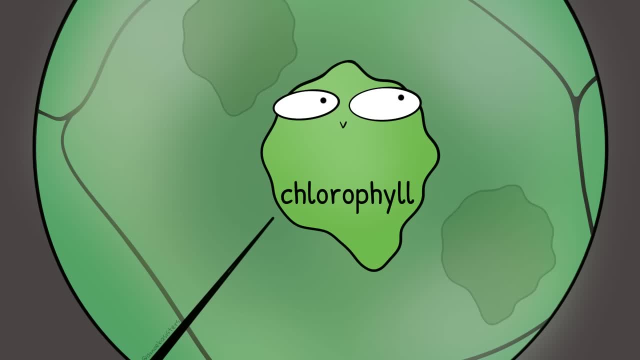 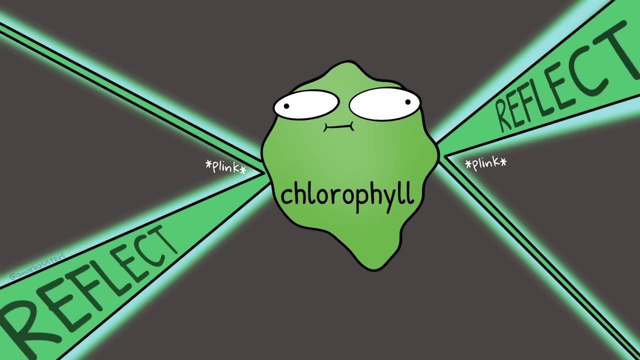 So a pigment that plants commonly use to capture light is called chlorophyll. Chlorophyll does a great job at absorbing red and blue light, but not so much green light. Chlorophyll reflects green light, resulting in many plants appearing green to our eyes. 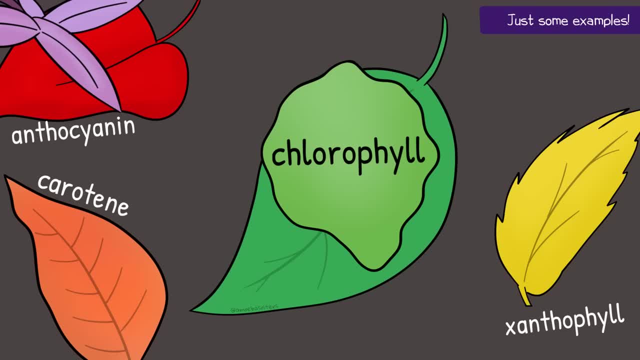 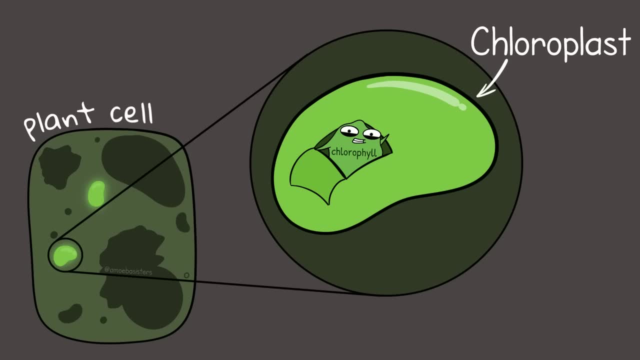 There are pigments besides chlorophyll. Chlorophyll works with different wavelengths of light, and this can explain why green is not the only color you see in plants. Chlorophyll is a pigment that can be found in the chloroplasts of plant cells. 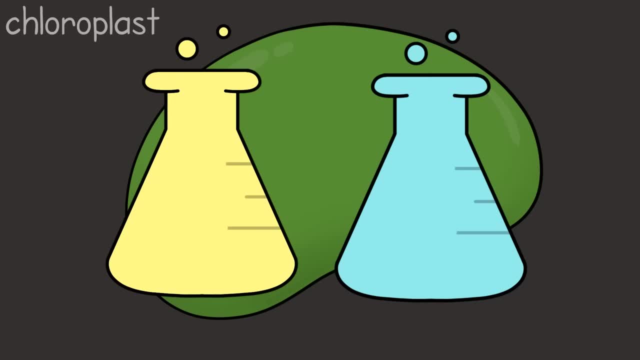 There are two major processes that occur in the chloroplasts that together make up photosynthesis. They are the light-dependent reactions and the light-independent reactions. The light-independent reactions can also be called the Kelvin cycle, or, even less commonly, 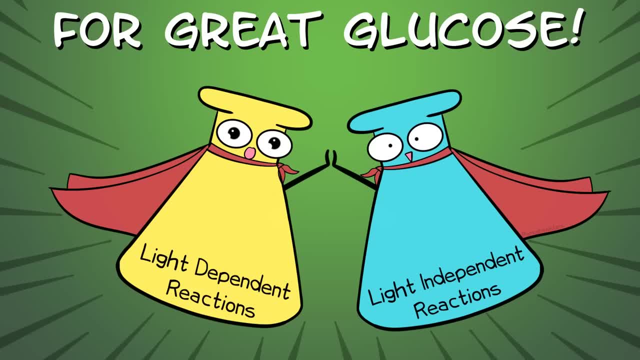 the dark reaction Sounds intriguing. We're going to talk about chlorophyll. We're going to talk about both of these briefly and please remember, like most of our videos, this is pretty general. We've got some further reading links in the video description where you can explore. 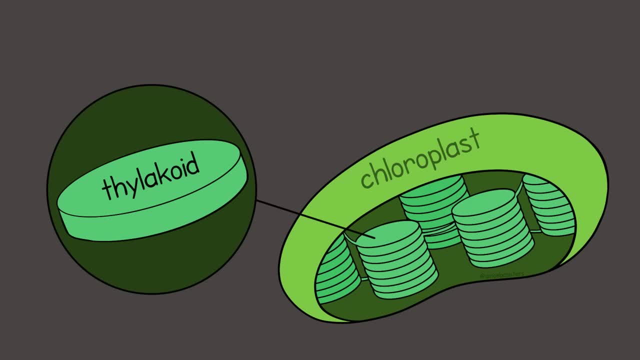 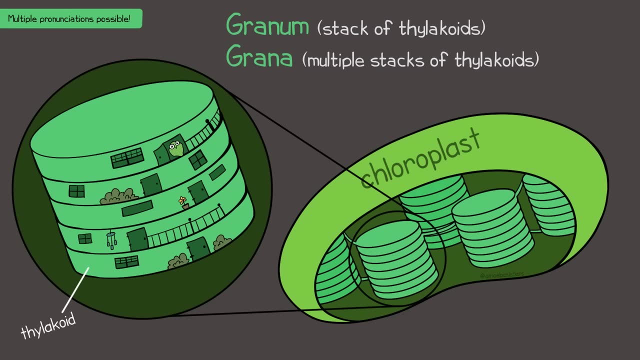 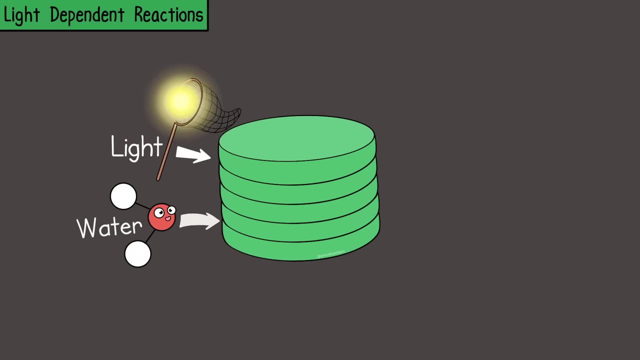 a lot more detail. So light-dependent reactions happen in the thylakoids, Little compartments in the chloroplasts that contain pigment. A collective stack would be a granum, Multiple stacks would be grana. In the light-dependent reactions, light is captured and water, which is a reactant in 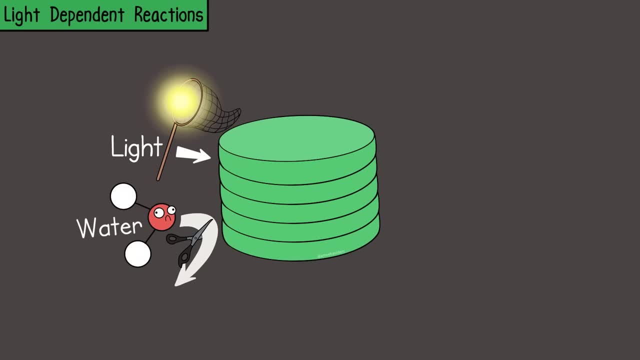 the photosynthesis equation is split. That means light is captured. That means, if you think of the chemical formula for water, which is H2O, it is split so you get electrons, protons and oxygen. So oxygen is also a product of the light-dependent reactions. 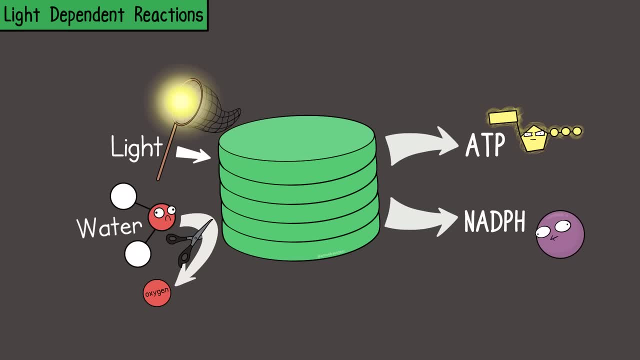 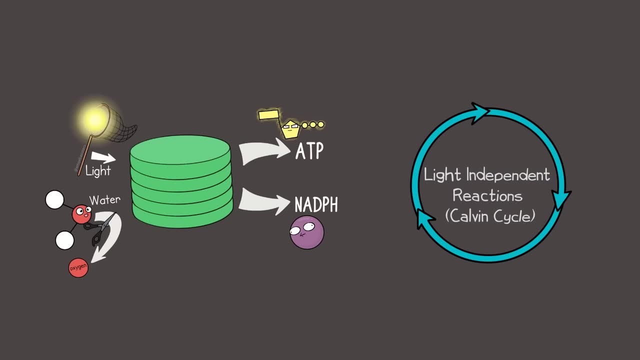 The light-dependent reactions also produce ATP and NADPH, which we'll get to in a little bit. Both the ATP and the NADPH will be needed for the next process, the light-independent reactions also known as the Kelvin cycle or dark reaction. 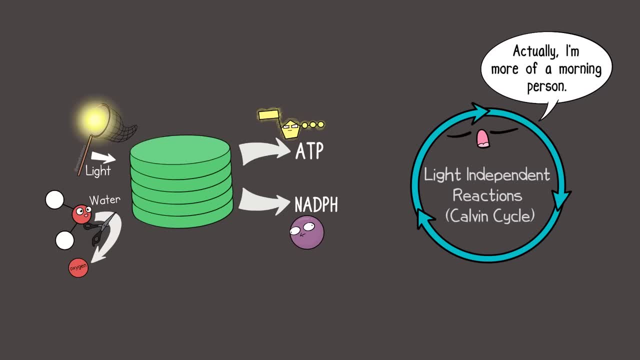 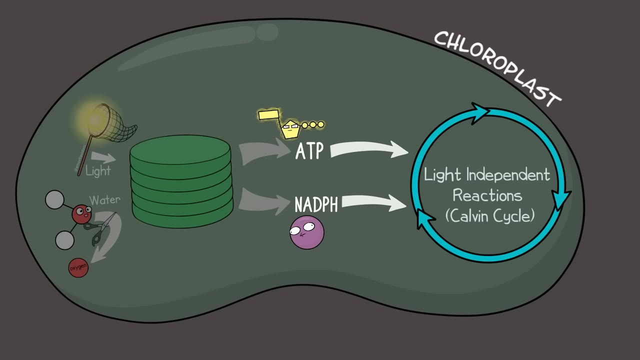 The name is a bit confusing. While, yes, the process isn't directly capturing light, it doesn't require darkness either, And again, it will need items from the light-dependent reactions like the ATP and NADPH. The light-independent reactions still happen in the chloroplasts, but specifically the 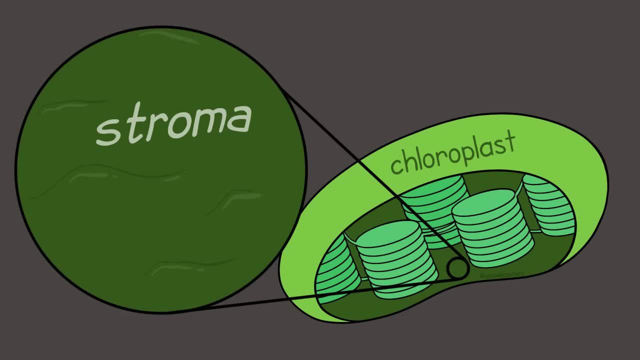 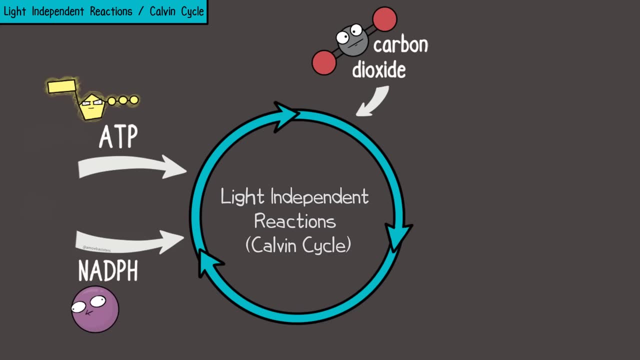 light-independent reactions happen in the stroma. The stroma is a fluid outside of the thylakoids In the light-independent reactions, or Kelvin cycle. chloroplasts are also called chloroplasts. Chloroplasts are also called chloroplasts. 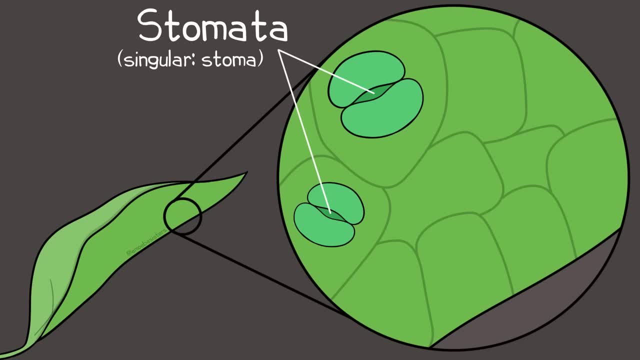 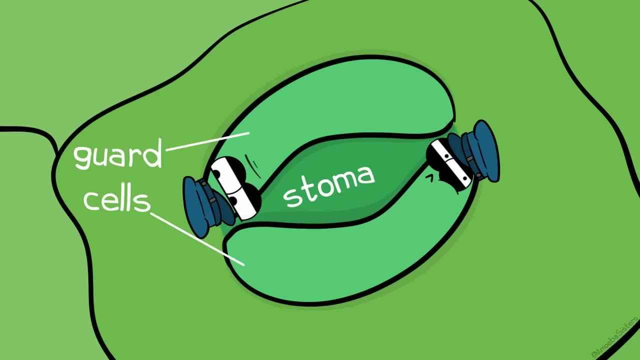 The carbon dioxide enters. It is taken in through pores that are often, but not always, on the bottom of leaves, And those pores are called stomata. Plants have the ability to open and close their stomata. The carbon dioxide gas enters the stomata and will be fixed. 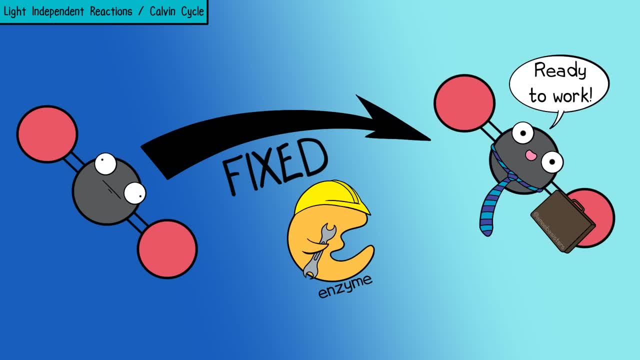 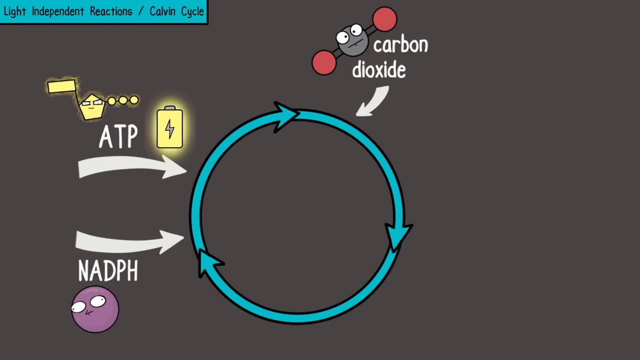 By fixed I mean that, with the additional help of a major enzyme, the inorganic carbon dioxide is changed to a more usable form. The ATP from the light-dependent reactions will act as an energy source. The NADPH will act as an energy currency for the Kelvin cycle. 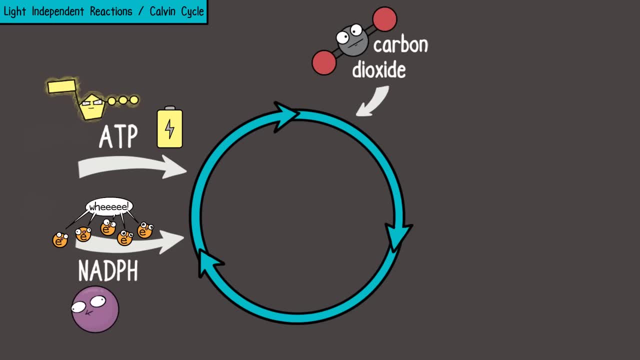 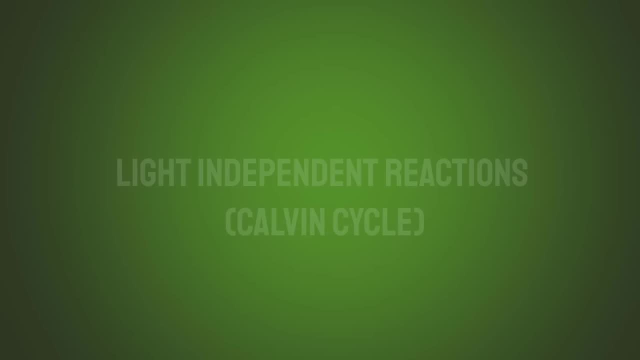 The NADPH that had come from the light-dependent reactions will supply, reducing power. By that I mean that it helps add high-energy electrons to this process. So in a very complex series of pathways, the fixed carbon dioxide, ATP and NADPH are used. 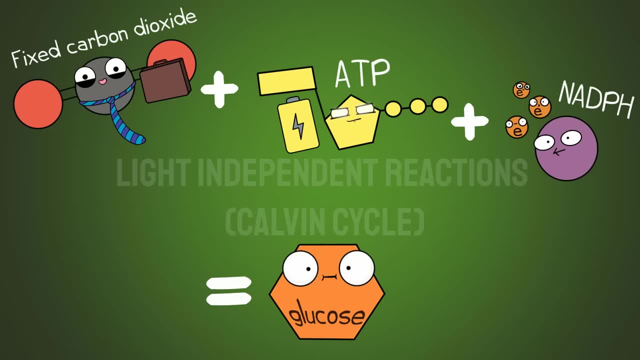 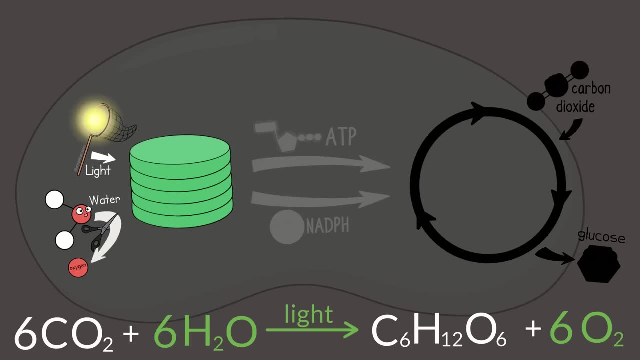 to make a product that ultimately can be converted into glucose, A sugar. So let's take a look at this equation. Last time I promise. So we have here the NADPH. Then we have the circled items. These were from the light-dependent reactions. 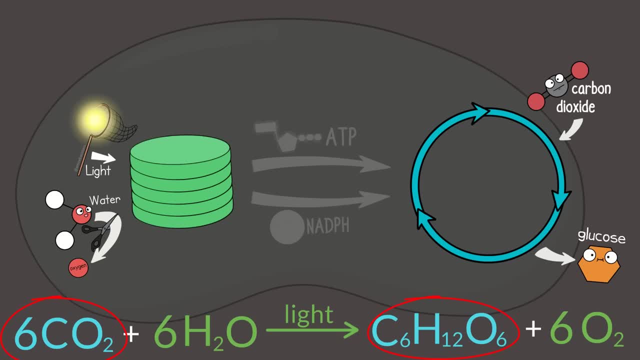 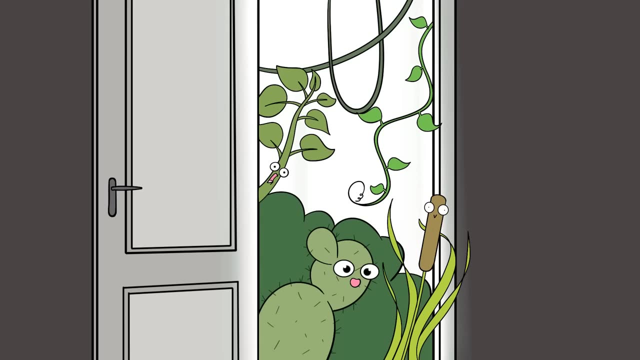 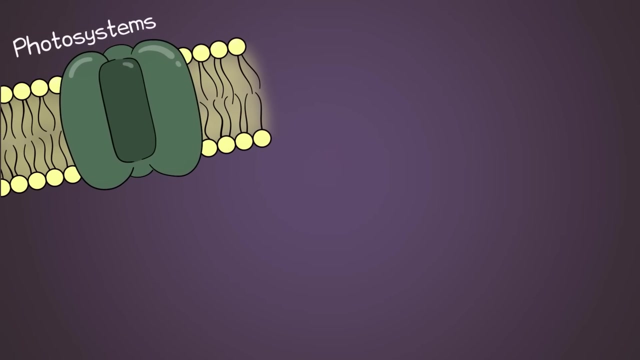 Now notice these other items: the carbon dioxide on the reactant side and the glucose on the product side. Those were from the Kelvin cycle. Remember, there is so much more detail to explore in this amazing process. You can learn about the photosystems that are in light-dependent reactions, or detail. 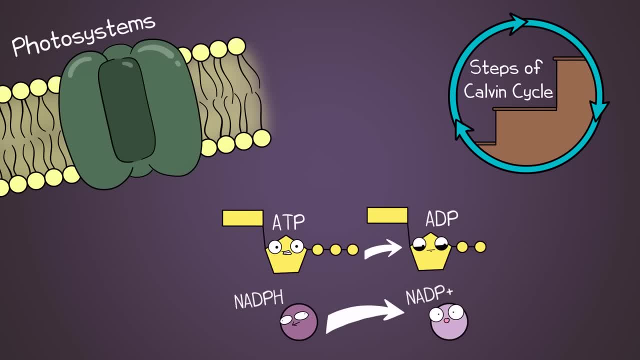 of all the steps in the Kelvin cycle And how ATP and NADPH will be converted into glucose. We have the carbon dioxide on the reaction side. NADPH will be converted to ADP and NADP+, which can then be used again by the light-dependent. 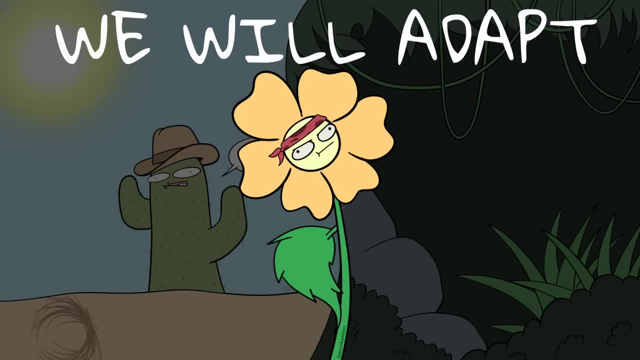 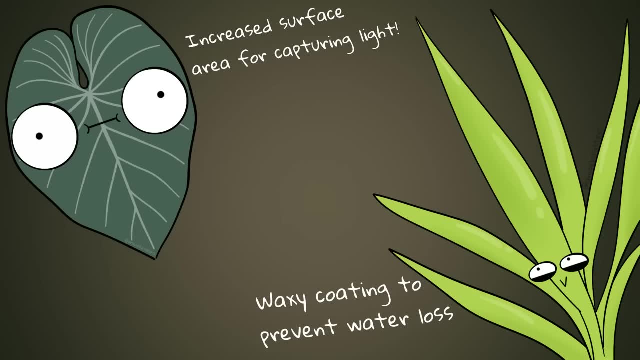 reactions. But before we end our short video, we do want to mention that plants have some amazing adaptations that can help them perform photosynthesis efficiently in very different environments. Many of these adaptations can involve the diversity of leaf shapes, coverings and pigments. 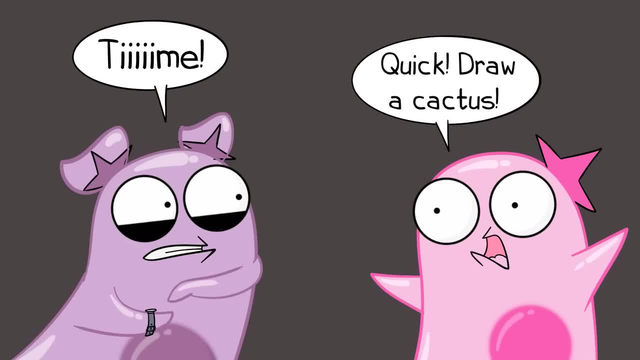 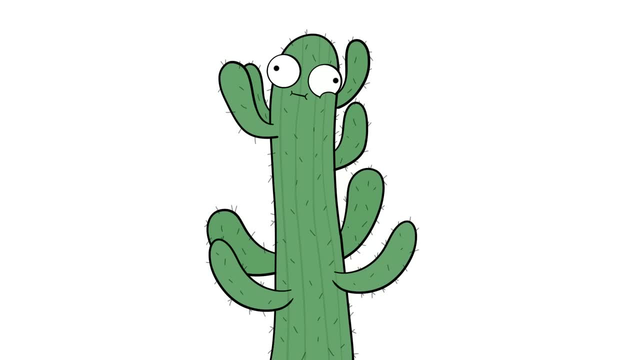 This is definitely worthy of a completely separate video topic, but just to give a neat example of an adaptation involving photosynthesis, consider the cactus. Cacti have a potential problem. They often live in a hot desert, and so if they open their stomata during the hot day, 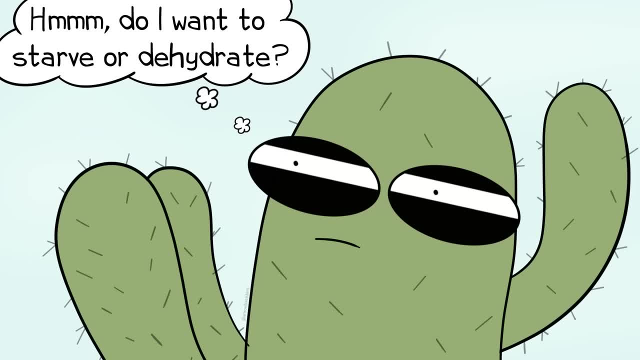 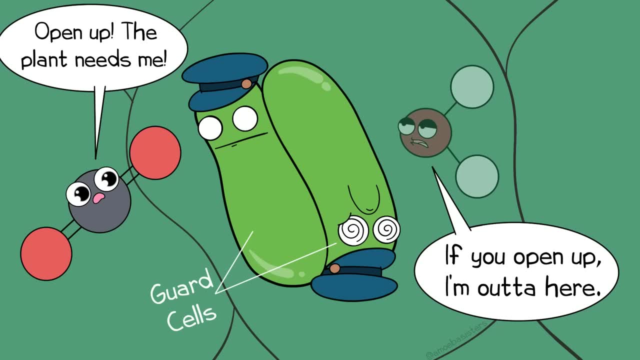 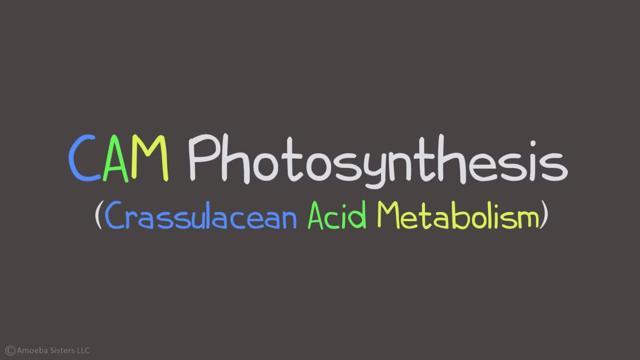 to get their carbon dioxide. they can easily lose more water than would be ideal. The precious water can escape through the stomata if the stomata are open, and that will happen at a faster rate in the hot desert sun. But cacti and some other plants too can do something called cam photosynthesis. 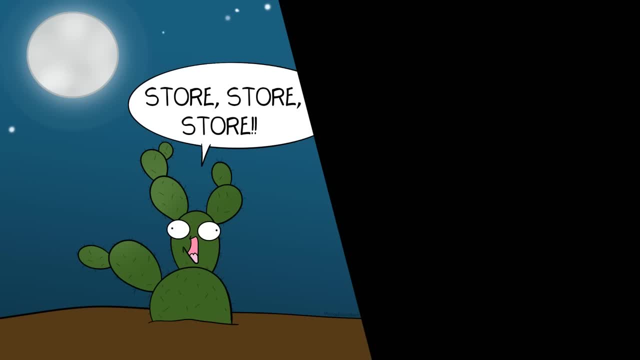 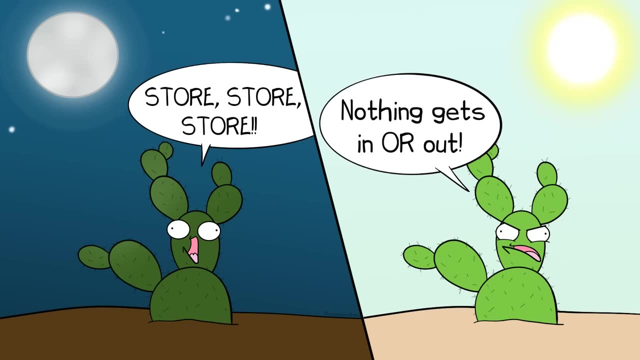 In cam. photosynthesis Plants can open their stomata at night, when it's not so hot, and they can capture carbon dioxide and chemically store it. They can then use this carbon dioxide the next day when the sun is shining, and yet